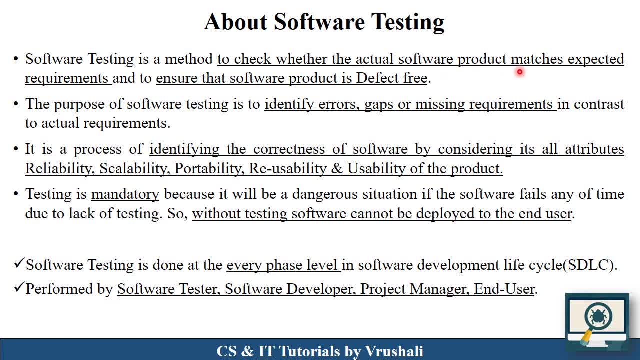 product or actual software product is developed as per the customer requirements or not. Basically, they ensure that your software product is completely error free or defect free. The primary goal of software testing is to identify all the errors, bugs, gaps or some missing requirements. 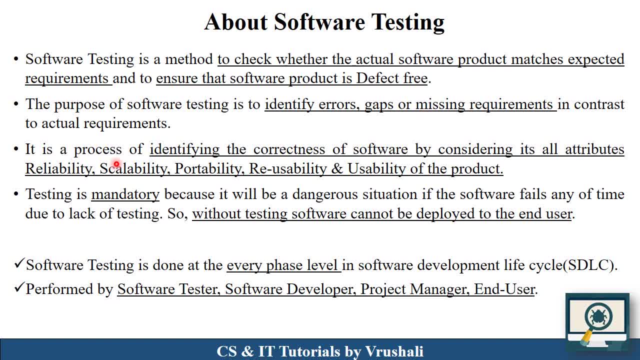 in your project. As per the definition, software testing is a process of identifying the correctness of software as per their reliability, scalability, portability, reusability and usability of the particular product. Software testing is one of the mandatory phase in software development life cycle. 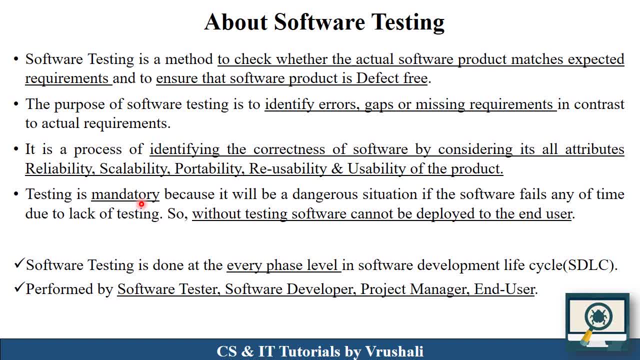 because they find out all the errors, bugs, defects in your project or program. So before deploy or delivered product to the customer, software testing is the primary and biggest task, one of the most important phase. this phase performed by the software tester, software. 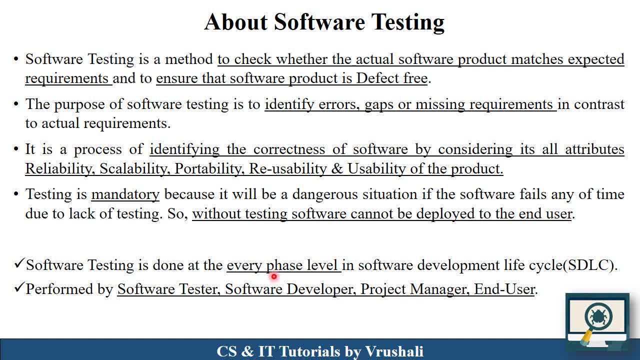 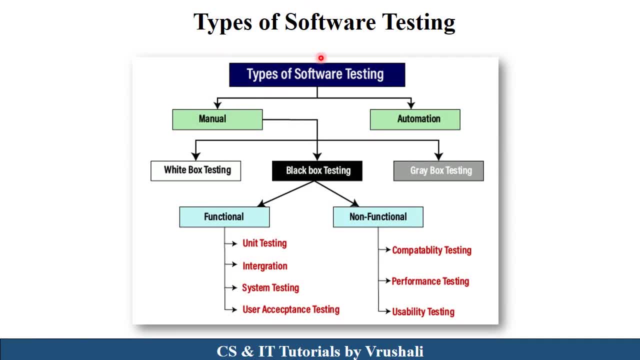 developer, project manager and end user at each phase of software development life cycle. now the next point is types of software testing. basically there are two types of software testing, like manual testing and automation testing. manual testing have divided into the three types: white box, black box and gray box testing. now black box testing divided into again two types: functional. 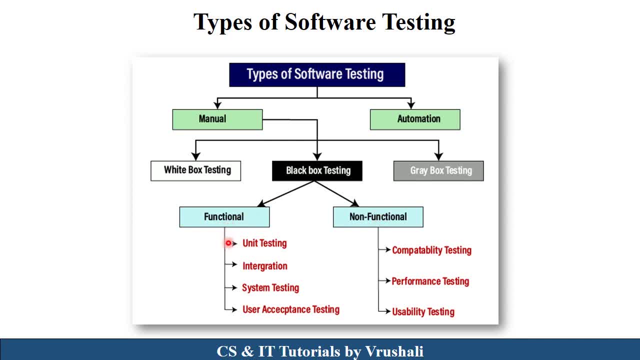 and non-functional testing. functional testing, again divided into the unit testing, integration testing system testing and acceptance testing. now non-functional testing, divided into the compatible testing, performance testing and usability testing. so these all are the types of software testing. we will discuss each type of testing with example from the next session. 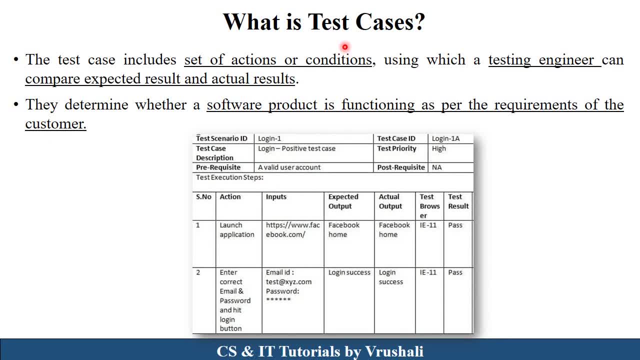 now the next point is: what exactly test cases? basically, test cases is a set of actions or conditions which is written by or generated by the tester. this test cases compare your expected result and actual result of your project. basically, it check that your software product is developed as per the customer requirements or not. see here in this diagram, this is a test case. 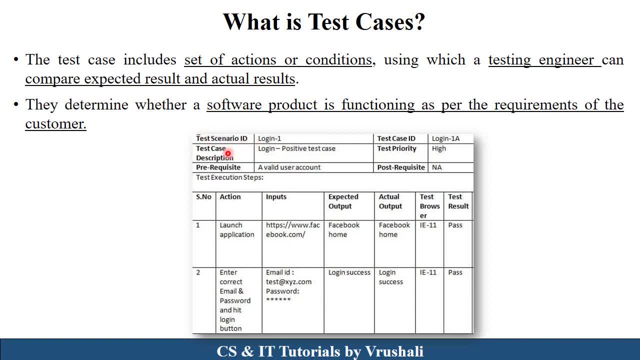 scenario. first there is a test scenario, id, test case description and prerequisite. see, you can use different types of applications or the product. now, always the first page is username or password. that is login page, right? so tester, read: write some different types of test cases for that particular. 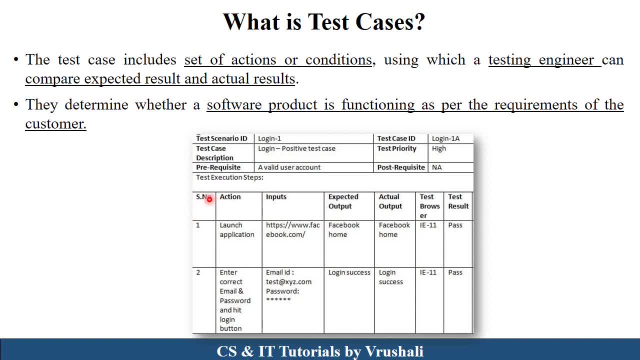 page. see here in this particular table, first there is a serial number. now next one is the action in action. first thing is a launch application, suppose the particular account of the facebook. okay, so there is a link of facebook that is facebookcom. now, expected output is when you click on this particular link: facebook home page. 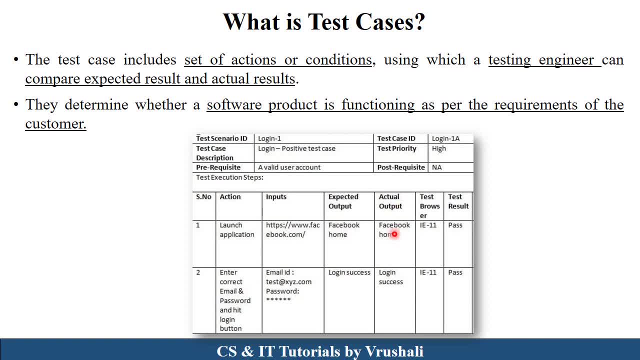 will be open. now actual output is also same. facebook page will be open. so your test result is pass. so in this way, they check that expected outcome and actual outcome of your project. similarly, when you enter email id or password- that is, username and password- and click on login button. so your input is this: this is: 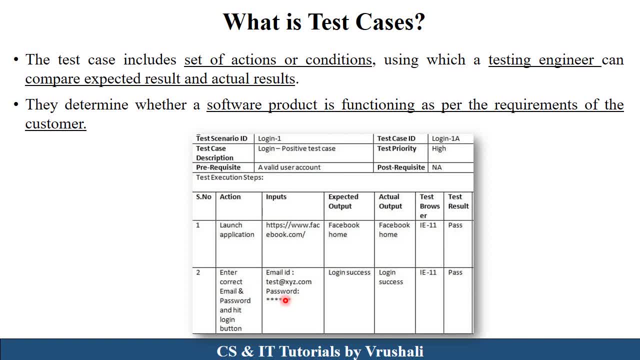 your email id and this is your password, if you enter correct password, so expected output is login successful. now they actually check that by entering username and password. actual output generate and login successful means your test result is pass. suppose you have entered wrong username and password. now your login is unsuccessful. 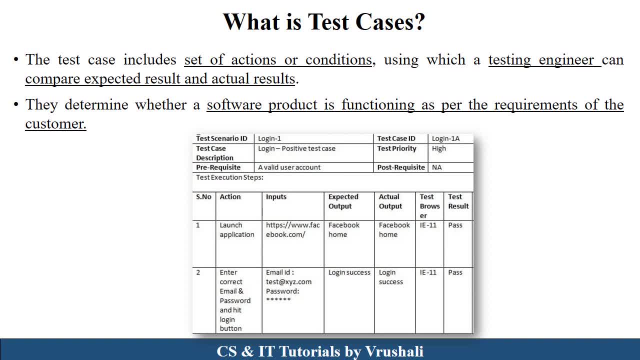 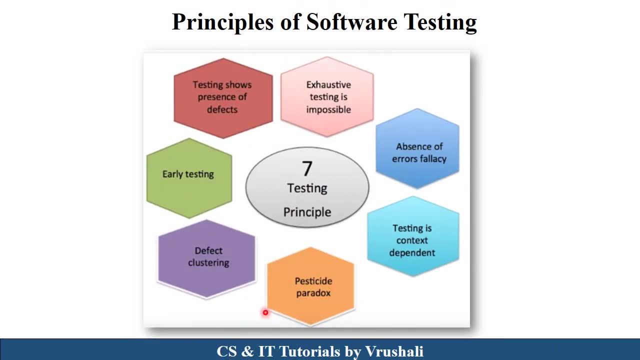 then test result is fail, so this is called as test cases. in this way, tester generate different types of test cases for each and every modules and functionality in your project. now the next topic is principles of software testing. there are total seven testing principles. let discuss each principle. 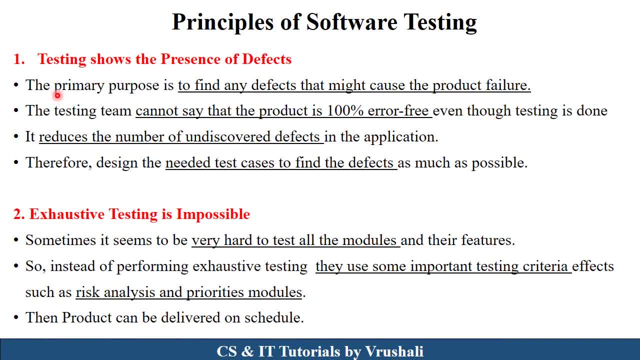 in detail now. the first principle of software testing is testing show the presence of defect. as we know, the primary purpose of software testing is to find out errors, defects, bugs in particular project. but after find out all those error, still tester team cannot say that your product or your 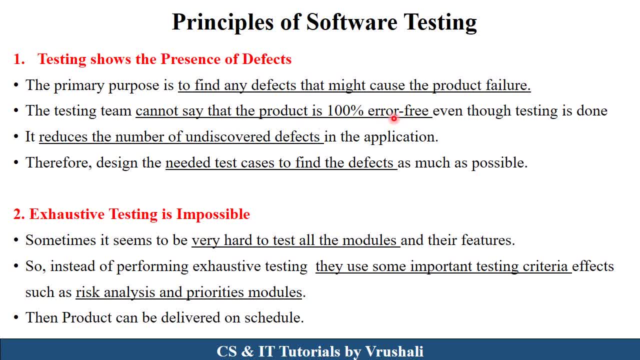 project is 100 error free. basically, tester just reduce the number of undiscovered defect. they reduce errors in your project. for that purpose, tester generate different types of test cases as per your product, as per the features of your project. the next thing is exhaustive testing is impossible. see, suppose there is a large scale project, there are different modules, are there? 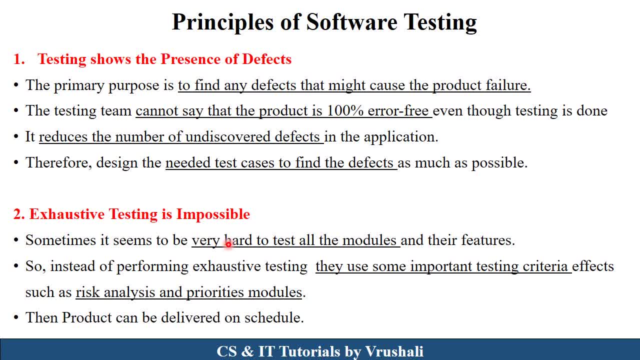 so to verify each and every module, each and every functionality of that module, it is impossible or it gets too much time right. so at that time tester focus on some important testing criteria, that is, risk analysis and priorities module. whatever the risk have generate in particular project, tester solve this risk problem first, after that priorities module, for example, suppose 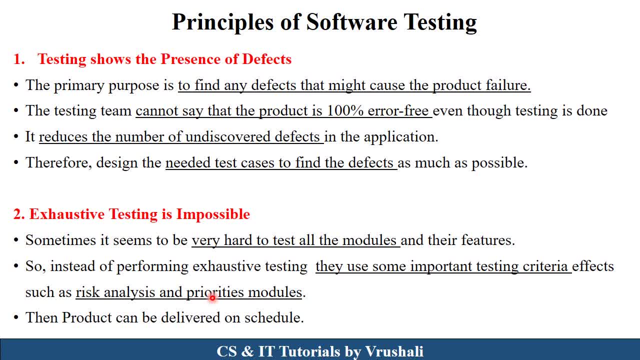 customer want module 1 and module 2 first. after that they want module 3 and module 4. so developer delivered module 1 and module 2 to the customer. this is a priority module. so tester check priority module first. that is a priority module. so tester check priority module first. that is a priority. 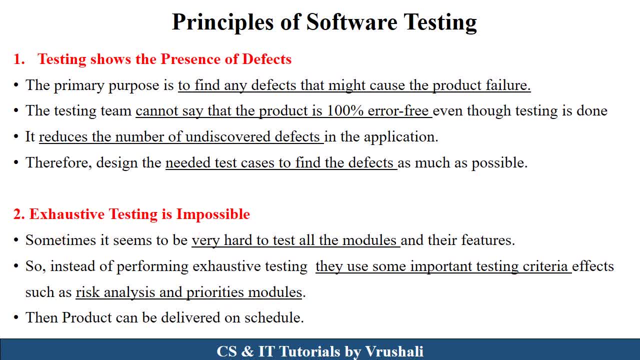 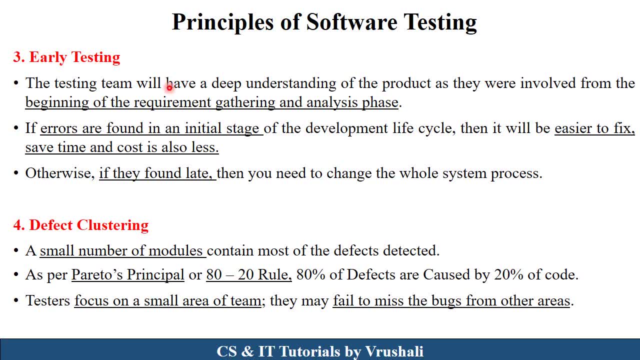 that's why exhaustive testing is impossible. they focus on main testing criterias. now the next principle is early testing. as we know, in software development life cycle the first phase is requirement gathering and analysis phase. so tester involve in particular product or involve in particular project from the first step of software development life cycle. tester understand your. 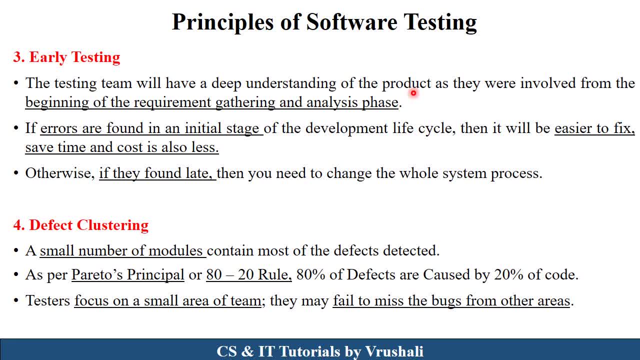 complete product, your complete project very deeply. understand your complete project very deeply. here suppose any errors are find out it initial stage of development life cycle, so that is very easy to fix. they save time and cost is also less. but if the errors are found, to find out a delay or 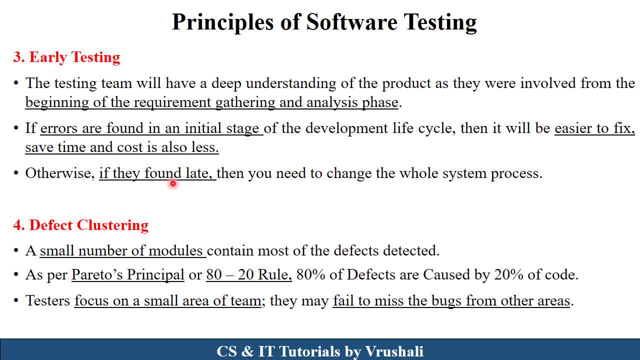 after, at the time of delivery of the particular project. so as a team, there is a need to change hold system process now. a next one is a defect: clustering- see in particularblicit customer policy obligatory hate network, such brown line. where, example, this code slightly differs from the mechanism that during hundred 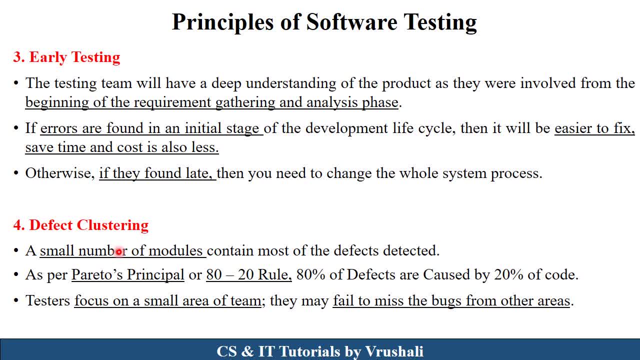 across point of the two master block argument and created and so on. and so we are entering them to gone problems anymore project. there are lots of small modules. lots of features, functionality and specifications are there right. so this small number of modules are called as cluster. now, this small number of modules constant most of the defects or errors. 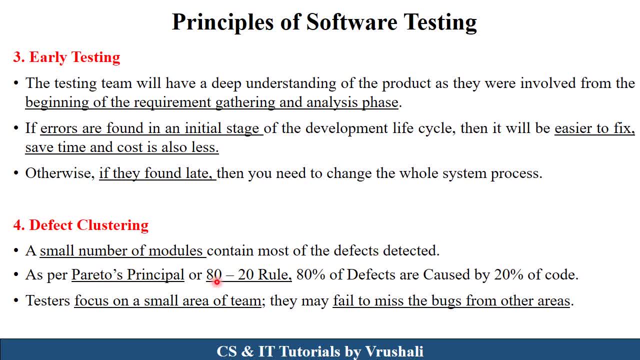 have detected. for that purpose, tester use Pareto's principle or a 2 to 20 rule here. as per that rule, 80% of defects are caused by 20% of code. this is a particular analysis by the tester. that's why tester focus on the small. 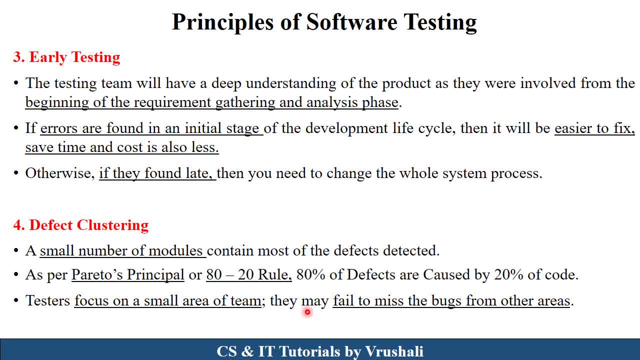 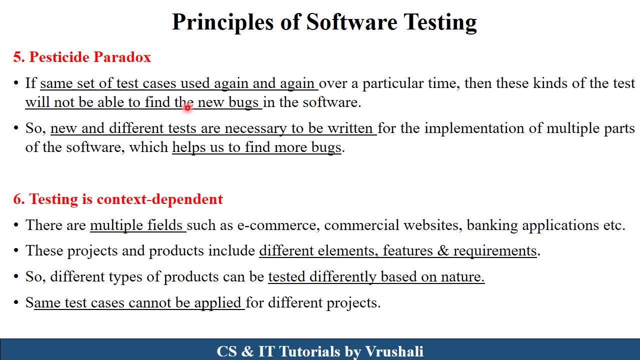 module or small functionality, small area of team, but the disadvantages of that: tester may fail to miss the bugs from the other area or other large applications. now the next principle is pesticide paradox. see as we discussed earlier. tester rewrite different types of test cases for particular product or 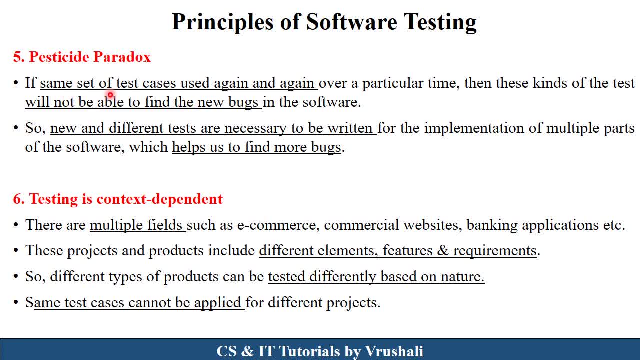 particular model but tester applies same set of test cases again and again. so at that time tester will not be able to find out any new bugs. so at that time tester generate or write some new and different test cases to find out different or new bugs in particular product. the next principle is: testing is context dependent, see 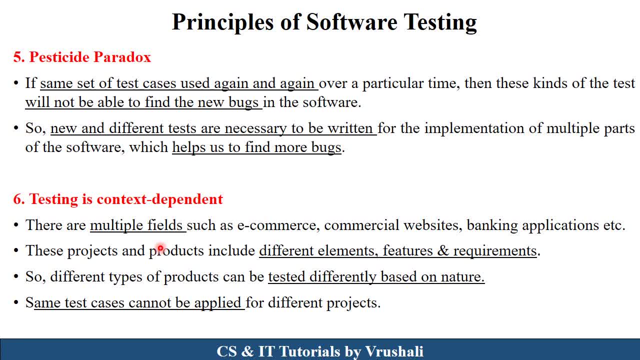 there are multiple fields, some web development projects, some app development projects are available, which is related to the e-commerce, commercial websites, banking application, Hospital application. so various types of products are available, every product, every project having different elements, different features and different requirements. right, so tester can't use same type of test cases to each and every. 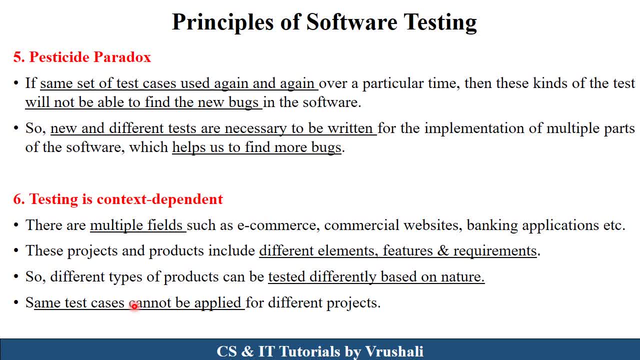 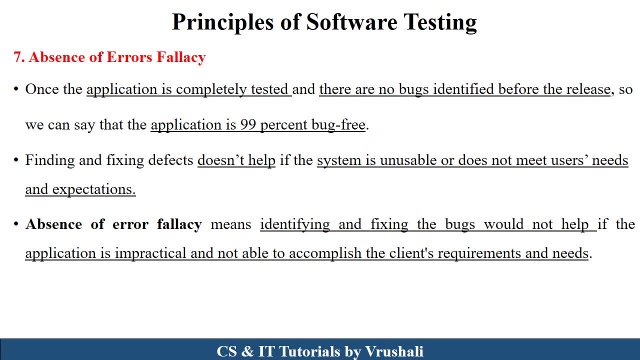 product. at that time, tester generate different types of test cases as per the nature or as per the feature of particular project. that's why testing is a context dependent test dependent. now, the last principle is absence of error fallacy. so absence of error fallacy means see after developing a particular product before deploy it to. 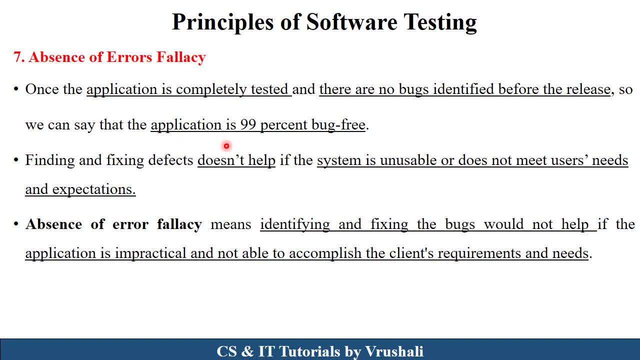 the customer. it check that your application or your project is 99% bug-free. but sometimes what happen? a particular project is not developed as per the customer requirement or as per the need of the customer. your project is unusable at that time. so this finding and fixing defects doesn't help. this is